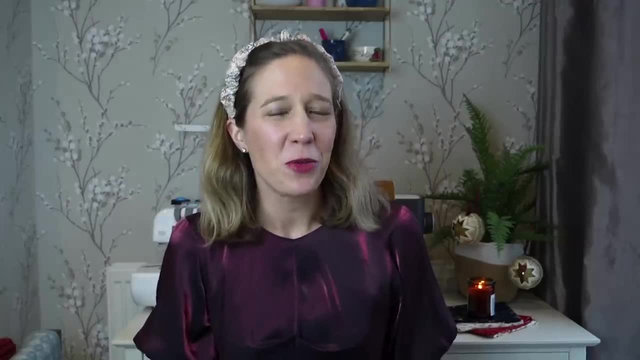 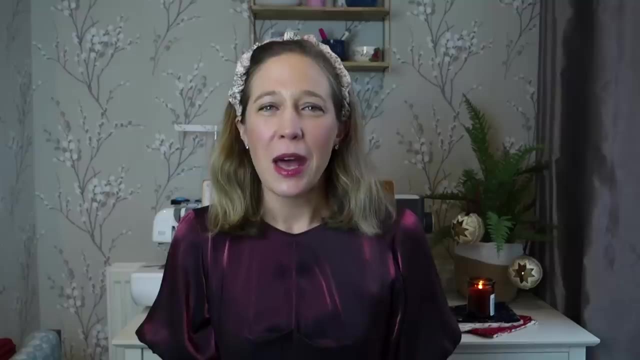 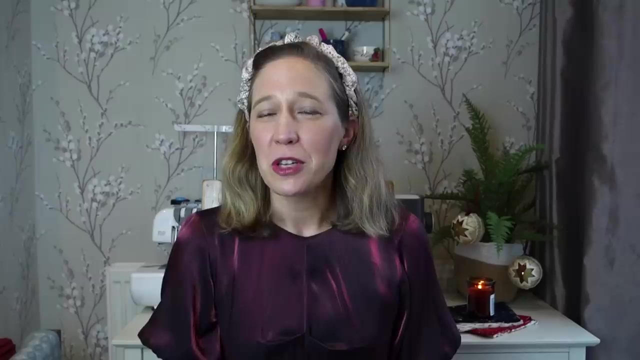 Hi, I'm Amelia and I'm so excited to share today 10 great ideas for handmade gifts. Hi, so I'm Amelia and this is my channel, Sew Amelia, where I share lots of ideas about making a handmade wardrobe for me and my children. Today, however, I'm going to be sharing 10 ideas. 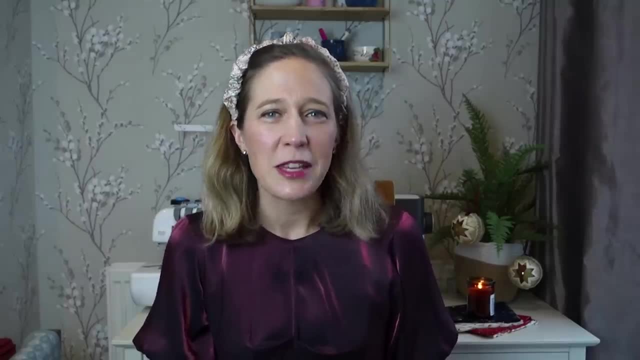 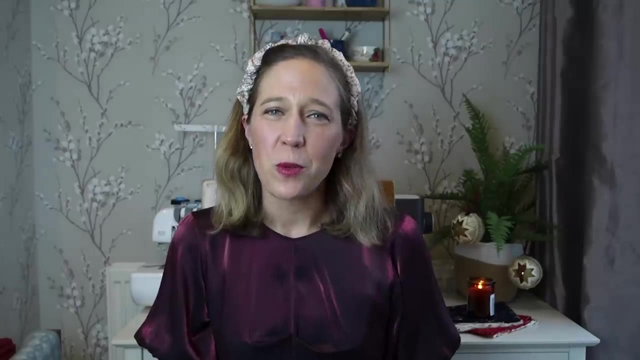 for handmade gifts. These could be for Christmas, they could be for birthdays, they could be for any time of the year, and I hope you'll enjoy watching as I share these ideas with you. So I'm sharing these ideas today as part of the vlogger tour for the. 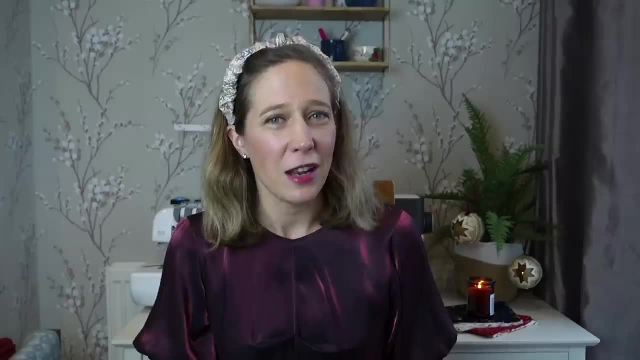 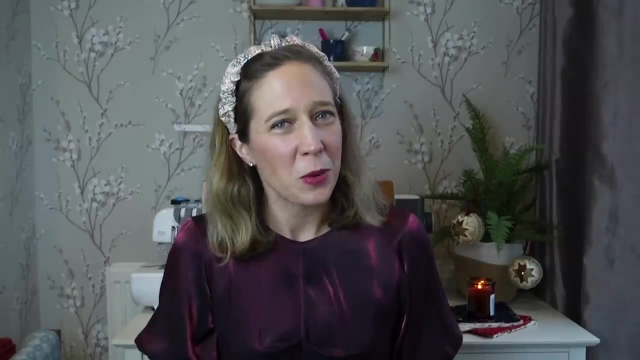 wonderful challenge: A Gift to November which is being hosted by Alison, who's Sew Like Dottie, and Adam, who's Adam Sews. So the idea behind this challenge is to encourage us to get our gifts that we always want to make for Christmas sewn up before that December rush. So the idea is to try. 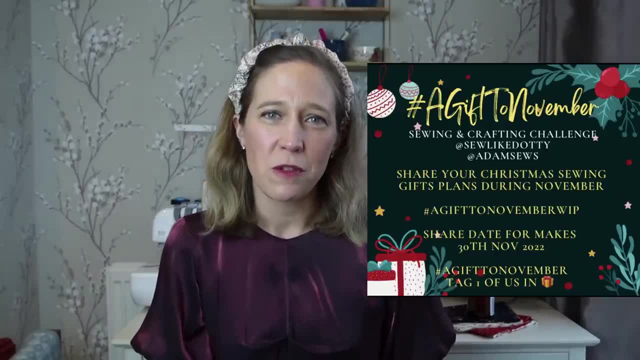 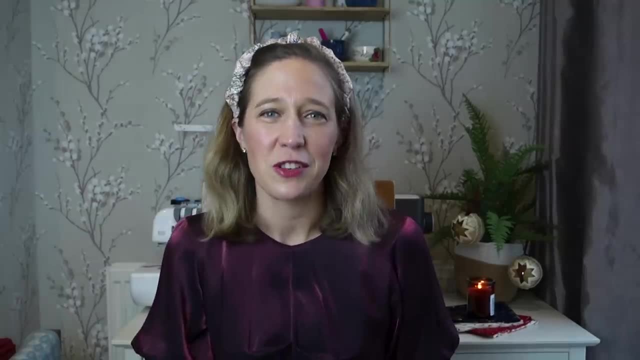 and get these made in November to share them on the 30th of November with the hashtag a gift to November. You'll be in to win some amazing prizes which have been donated very generously for this challenge. So you can make these presents for anybody yourself. 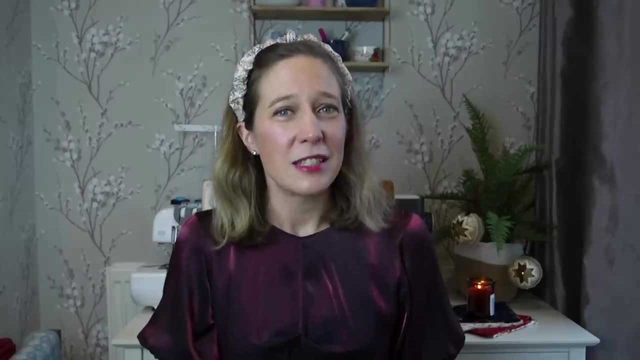 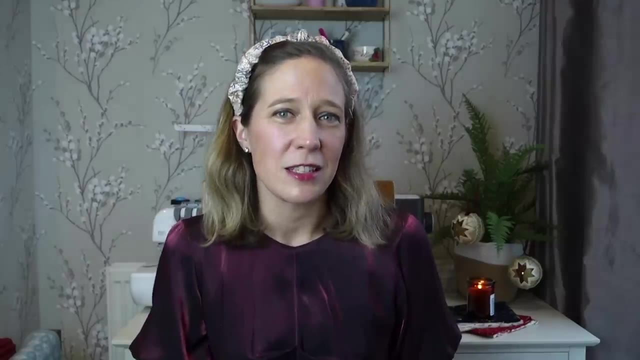 your friends, your family, your pets. The only rule is that it does have to be sewn or there has to be an element of sewing in the gift. So, with all that said, let me share my 10 ideas for handmade gifts. So the first idea I have which I'm super excited to get sewn up is the Hey June Handmade. 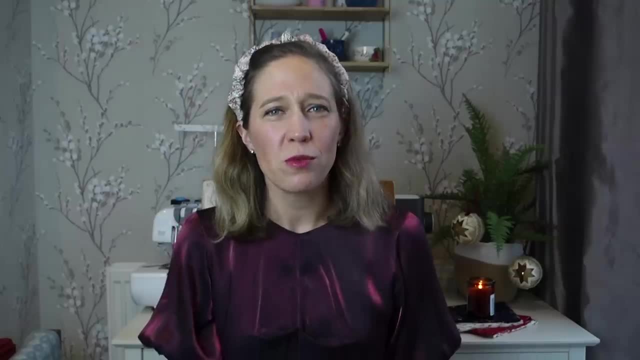 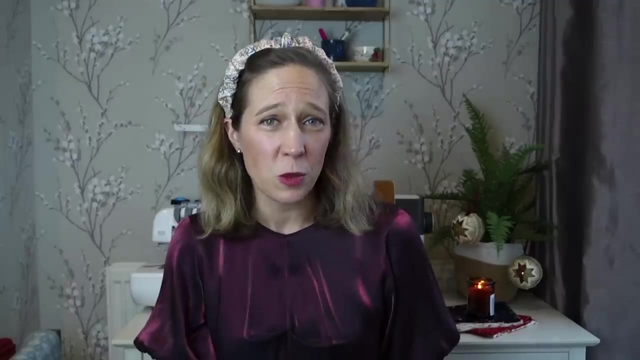 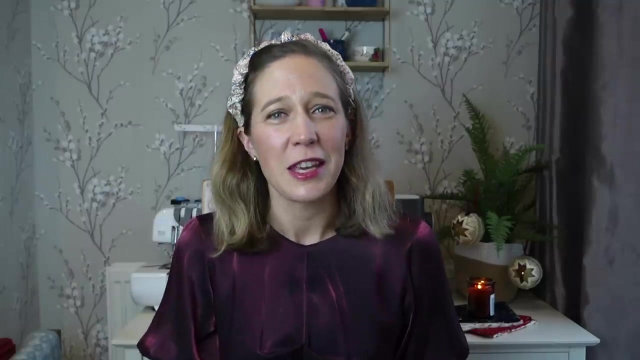 All Spice Apron. This is a free pattern for a really lovely looking apron and I'm sure there are lots of people in your lives that could use an apron either for working in the kitchen or in the living room. So this is a lovely pattern which just goes over the head and the arms go. 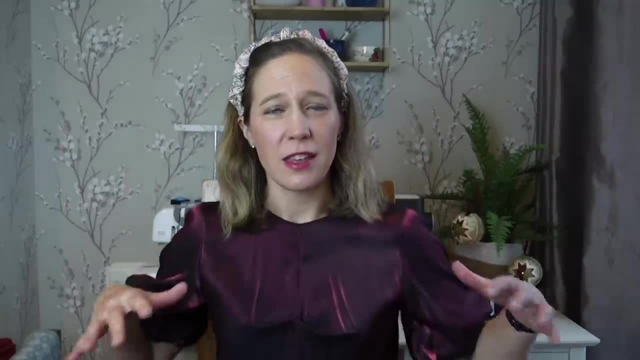 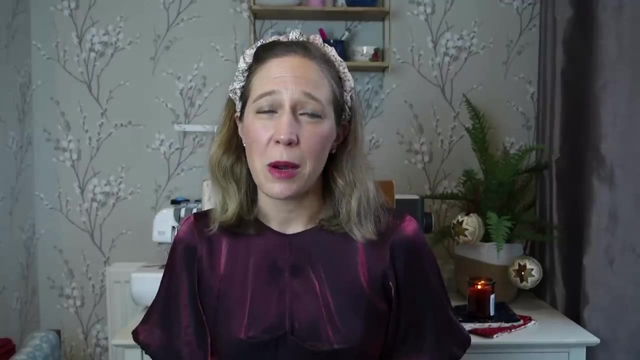 through. it wraps around and it just looks like it has such a beautiful shape. There's a big pocket on the front and the idea that I had was to perhaps put some embroidery on that pocket just to personalize this for the person I'm hoping to give this to. The other thing I like about this: 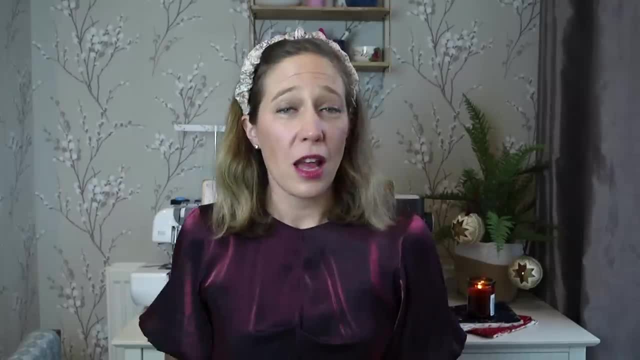 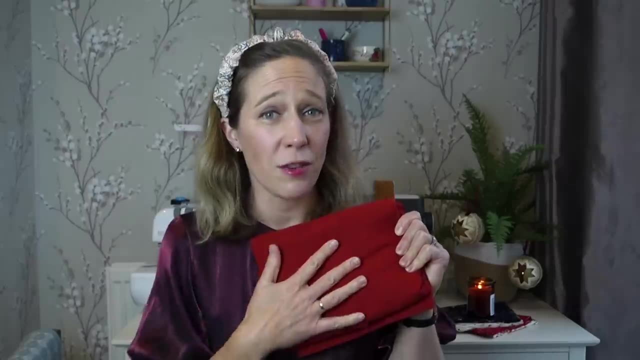 pattern is that it can be made out of a metre of fabric, and I'm sure we've all got fabrics in our stash that we could do with using up. In my case, I've got this beautiful viscose fabric that I've made out of a metre of fabric, and I'm sure we've all got fabrics in our stash that we could do with. 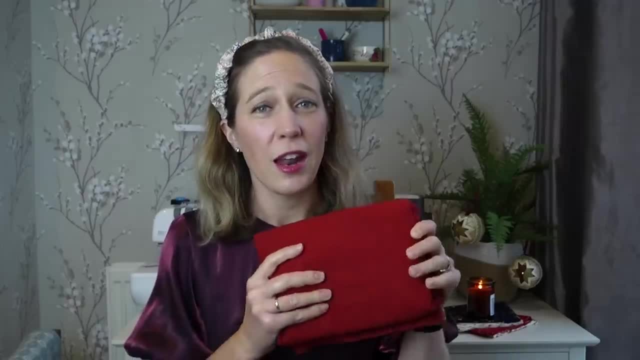 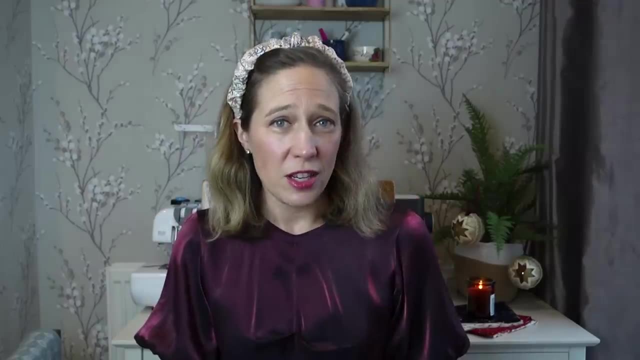 using up. In my case, I've got this beautiful viscose linen that I bought from Rainbow Fabrics so long ago, and I've just had a metre of it sitting waiting for the perfect project, and I think this might be it. So, as with all of the patterns that I mention in today's video, I will 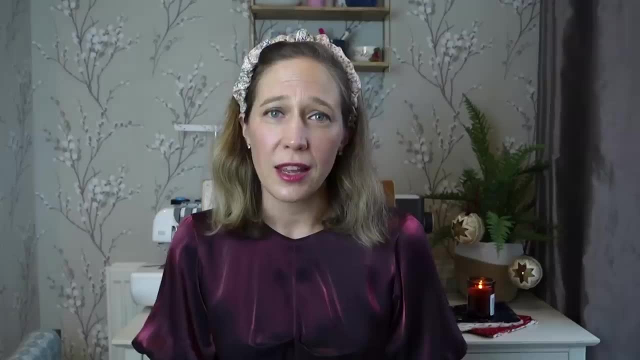 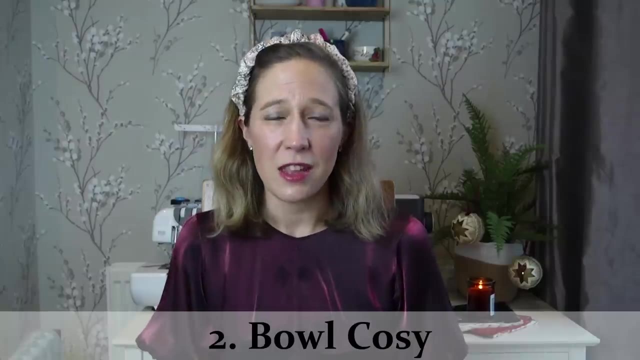 link everything down in the description box so that you can go and click on the link and take. it will take you directly to the pattern or to the page with the tutorial as I mention it in the video. So the second gift idea that I had is one that I have made before and that is a bowl cosy. 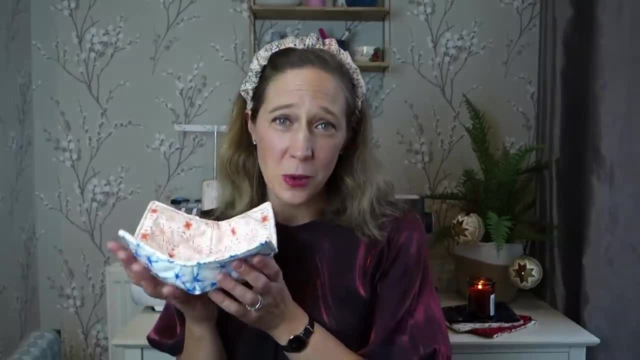 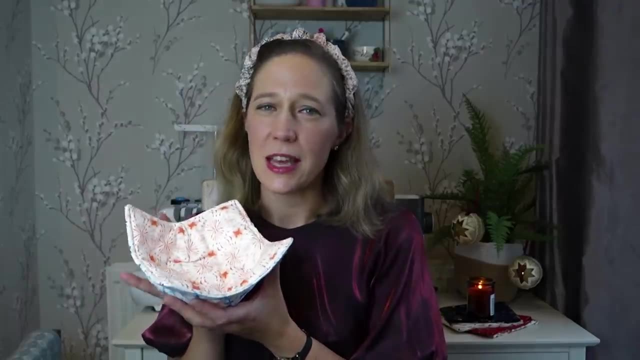 So I made these last Christmas and they were so quick to become together. I made them out of fat quarters from my Sew Hayley Jane box. Now, the only thing you need to be aware of when making these bowl cosies is that they do need to be made out of cotton. 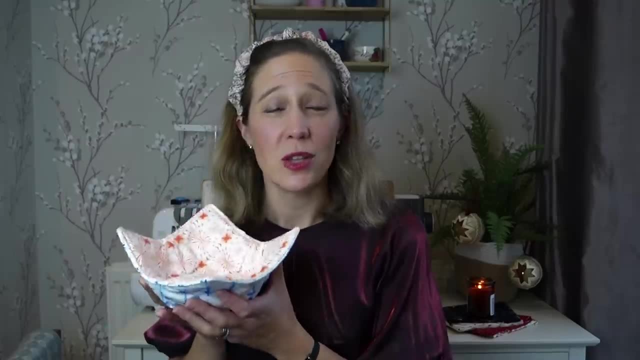 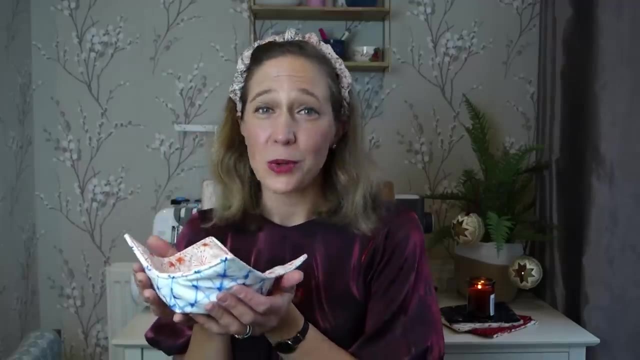 fabric and cotton thread and cotton wooding, because the idea is that you put them in the microwave with your porridge bowl or your soup bowl and then they keep your bowl cosy and your hands from getting burnt, which is perfect. Now the people I gifted these to have used them and used 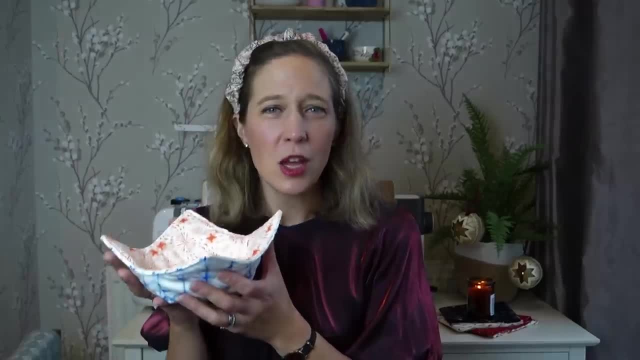 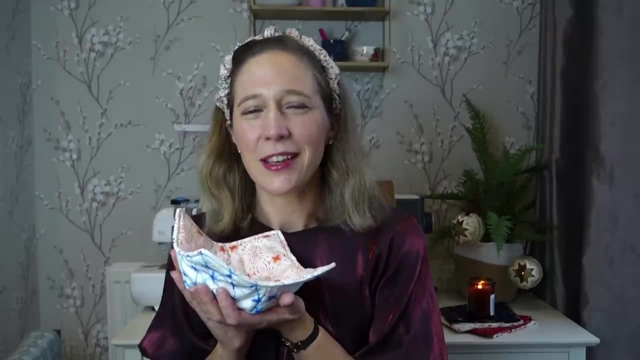 them and used them, and in fact I've used mine so much as well, not just for porridge and soup but for ice cream, because when you sit on the couch with a bowl of ice cream you don't want your hands to get cold, so I do also use it for that. So the bowl cosies come together really quickly and 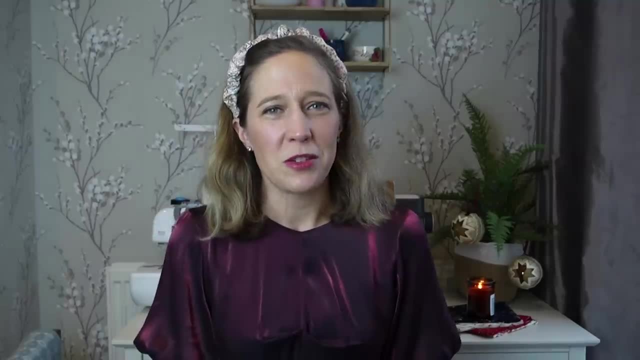 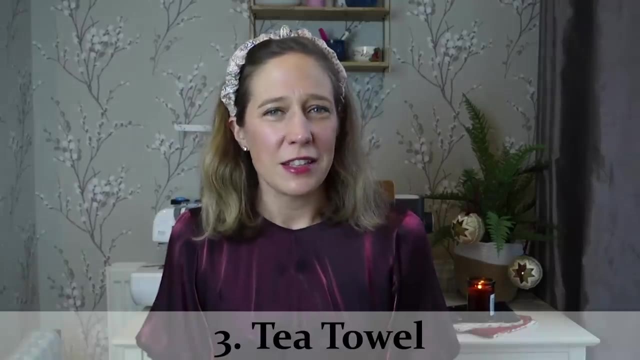 easily, and they're just a lovely little gift to either put in a stocking, perhaps, or to give to a friend that you know might use it. Now, the third gift idea I had for this year is one that I'd quite like to give to my children's teachers, and that is a tea towel. Now, I know that doesn't sound. 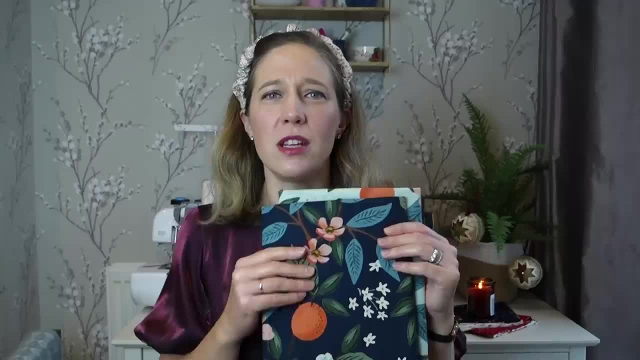 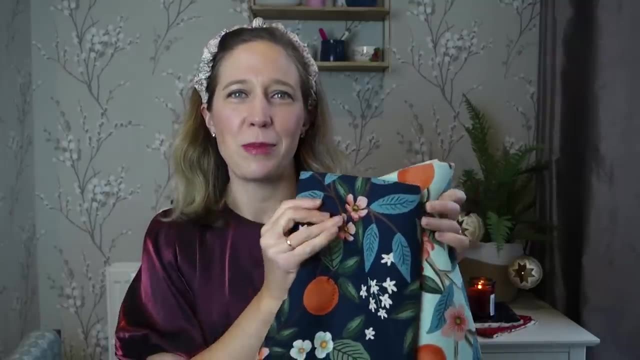 very exciting. but look at the fabric. So I found this cotton linen fabric over at System and Taka full paper cotton linen. It's in dark blue and also in light blue and I just thought a pair of tea towels like that would be gorgeous. And what I also saw on Pinterest was using a tea towel. 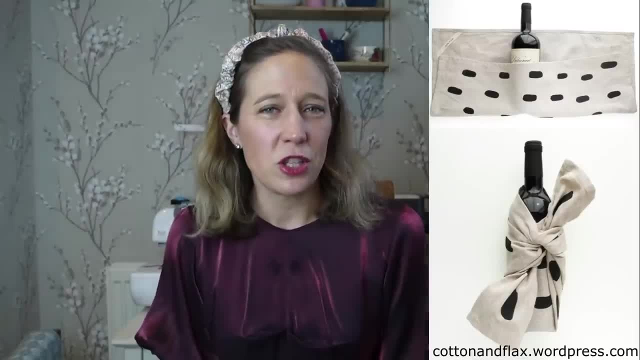 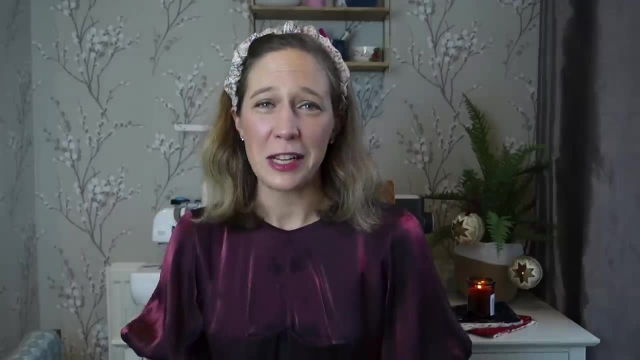 to wrap up a bottle of wine. So what I might do as a gift this year for my children's teachers is to make them a tea towel and wrap a nice bottle of wine in the tea towel so they can not only drink a nice bottle of wine but also really enjoy using the tea towel that it's wrapped. 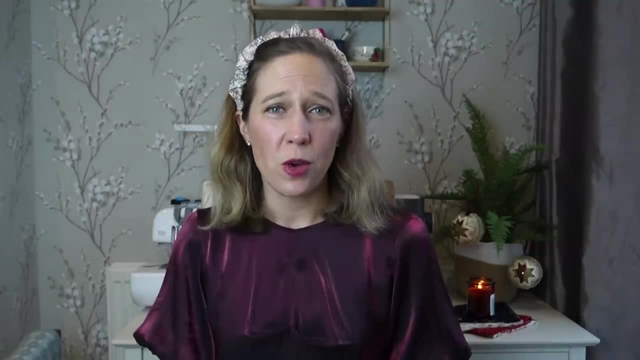 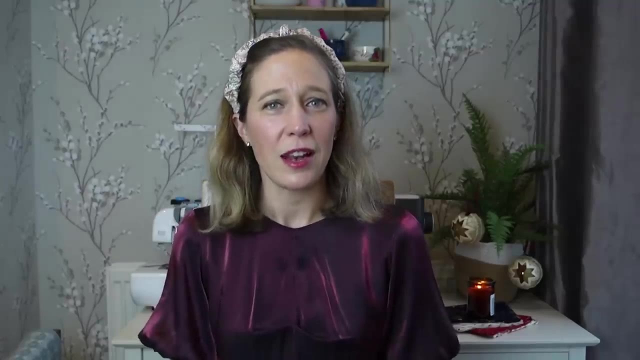 in Now. that's quite an easy project, but I have linked a tutorial below where it gave just really helpful ideas about the dimensions of the tea towel and also how to finish off the corners so they're mitered beautifully for that lovely finish. Now the fourth idea I'm going to share is another one that I've gifted to my children's teachers in. 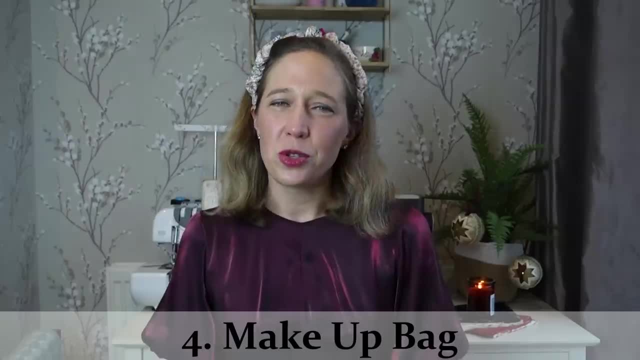 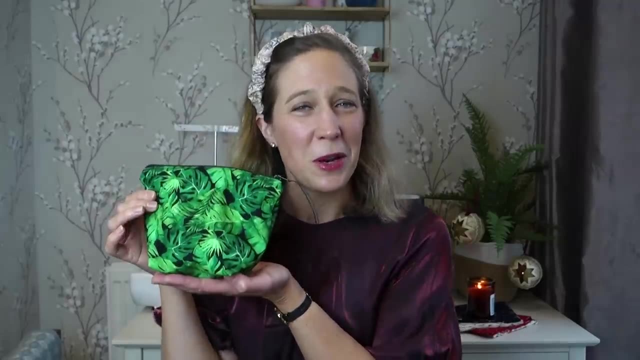 the past and that is a makeup bag. Now this is a tutorial written by Tamlyn, who has sewn on the tine for Sew Hayley Jane, and I'll link that again below. So here is one of the bags that I had left over, and what I put in it when I gave it to my children's teachers was a couple of bath bombs. 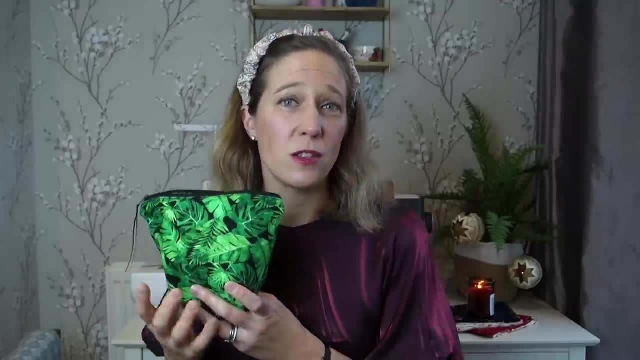 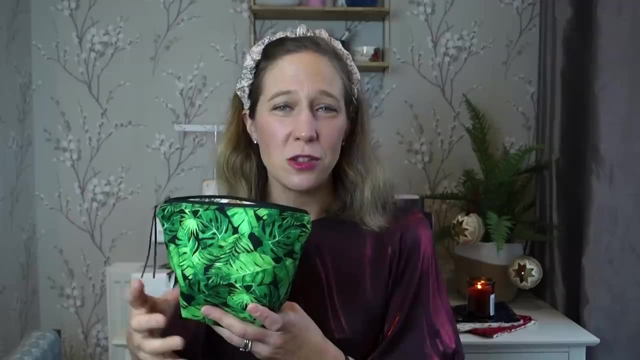 which I just thought was a nice idea. Now I've used these around the house for all sorts of things, not just makeup. We store technological gear in it for my children and for myself. We do put toiletries in here. we've put pencils and pens in here to use as a pencil case. They're so versatile. 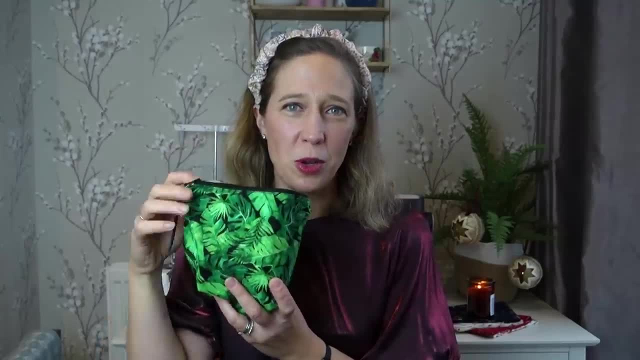 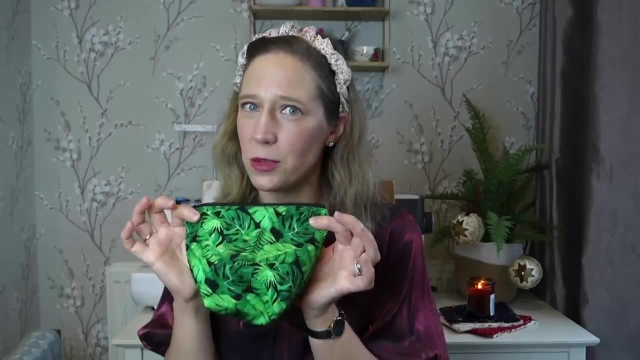 and I lined this one with such a cute pineapple fabric so you can use up lots of fat quarters that are in your stash or scraps of fabric. It's such a lovely tutorial to follow and it comes together super, super quickly. I think I batch sewed about nine or ten of these in a couple of hours. 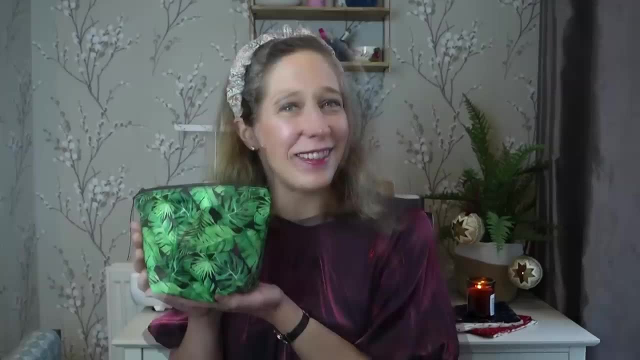 So that's idea number four: a makeup bag. Now I'm going to show you how to make a makeup bag. So I'm going to show you how to make a makeup bag. and it's another free pattern Now. keeping with the kitchen theme that I seem to have started with the tea towels, I thought another great gift would be. 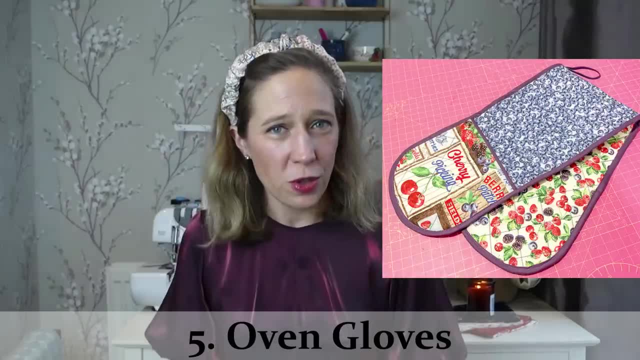 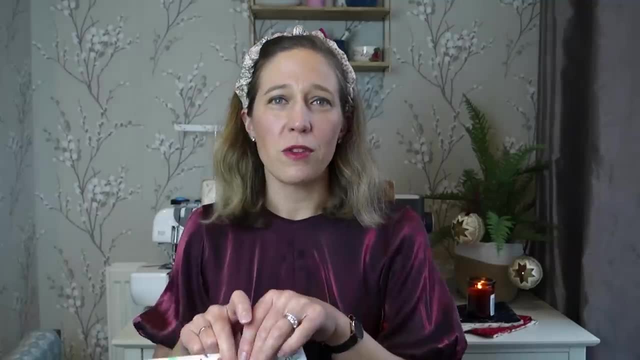 an oven glove. Now this is another free tutorial from Tamlyn, who is Sewn on the Tine, and you can find this over on the Sew Hayley Jane blog, And I've chosen three of the fat quarters that I got from a Sew Hayley Jane box, which have got macarons and coffee pots and things I think they would be. 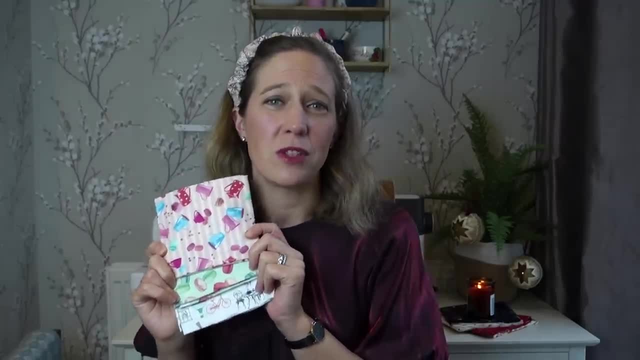 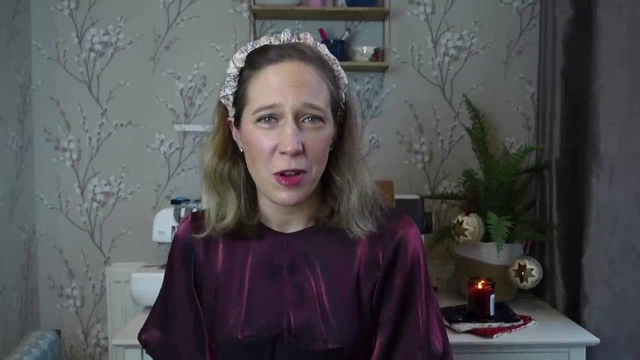 so cute in somebody's kitchen. And again, this is a great project for scrap fabrics because you could piece together different fabrics and you can use them in different ways. So I'm going to show you how to make it. You could use fat quarters that are in your stash, leftover scrap fabric, and I know. 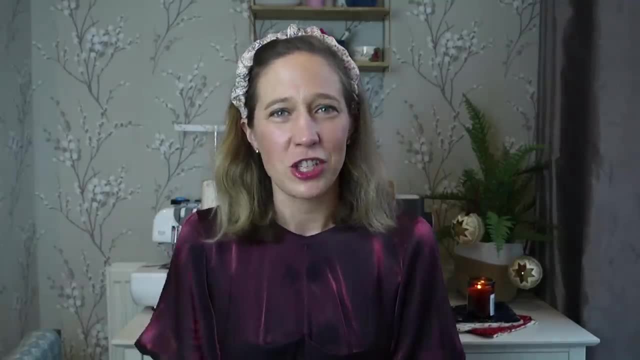 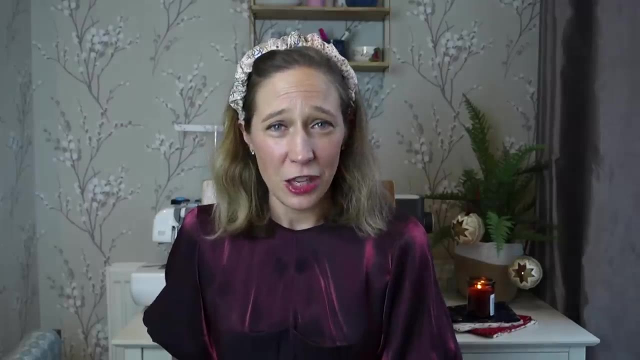 at the moment, we're all trying to use lots of things that we already have in our stash. I just think the oven glove would make such a lovely little stocking filler or a gift for a mother or a mother-in-law that might need one of these in their kitchen And the tutorials that Tamlyn writes. 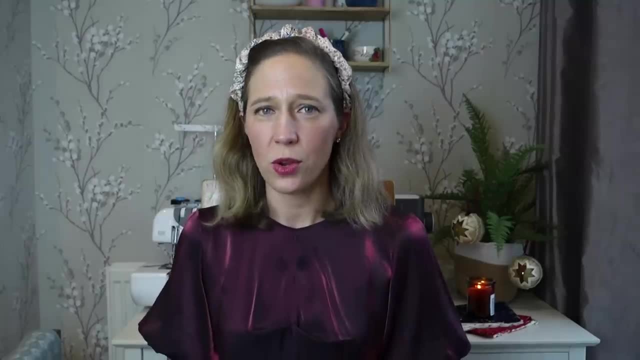 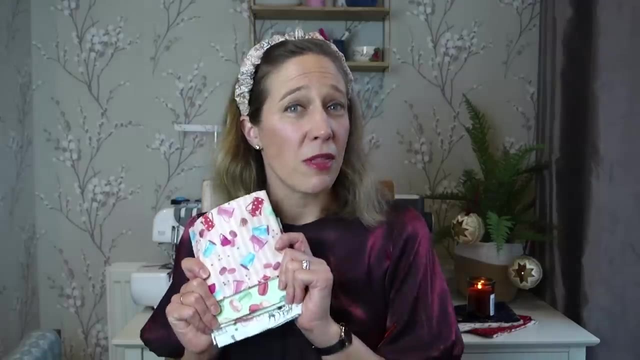 for Hayley Jane are so well put together, They're so easy to follow and guide you through step by step, and then you always end up with something that looks beautiful to gift. The only thing you need to bear in mind with this project is that you do need to use a special 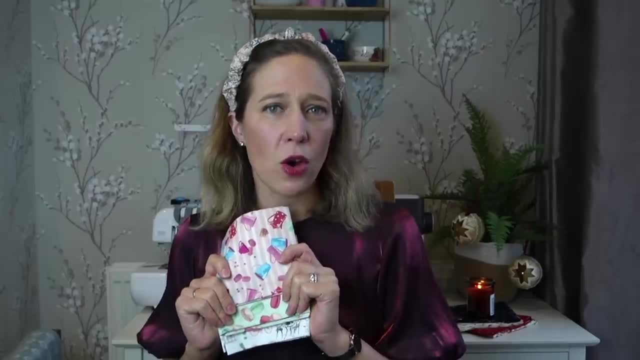 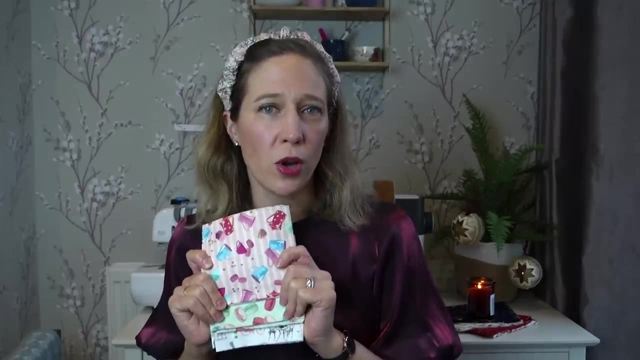 wadding that is heat resistant. There's a link on the blog for the type of wadding that you need and where to buy it. I do believe it's available from First For Fabrics. So do click on the blog link and double check before you start making this, as it's much, much better to make sure you. 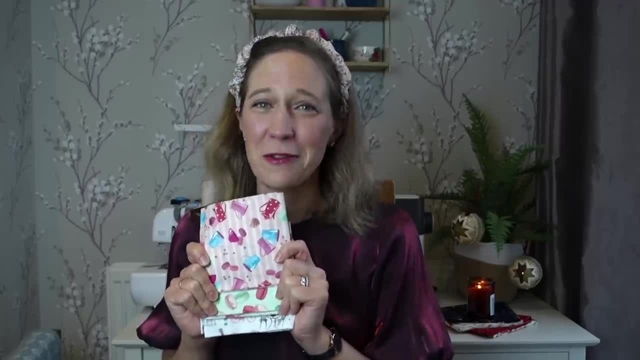 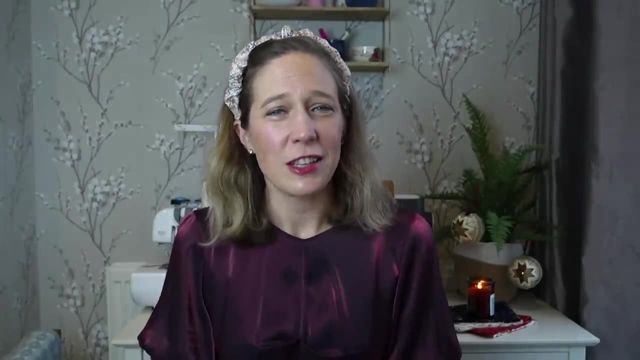 use the right wadding so that the person using the oven gloves stays safe. I've got three children and I do like to make handmade gifts for them and encourage them to make handmade gifts for each other. I just think it's so lovely to have a personalised gift made for you, and I also like 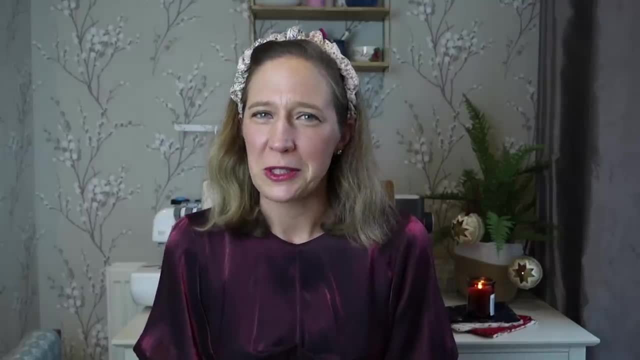 thinking about what they might really like to make. So I'm going to show you how to make a gift that they might like and enjoy, and making that for them to put under the tree. So something that I made for my children a couple of years ago now was hot water bottle covers. Now in the winter, 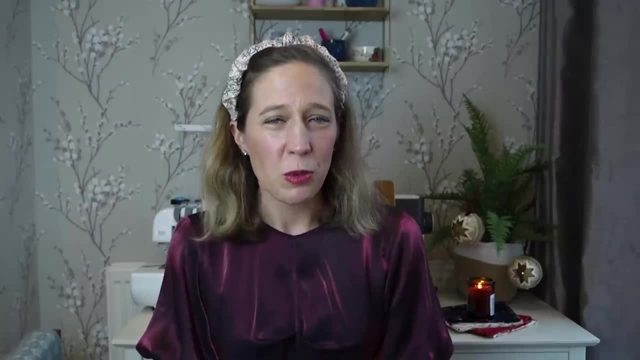 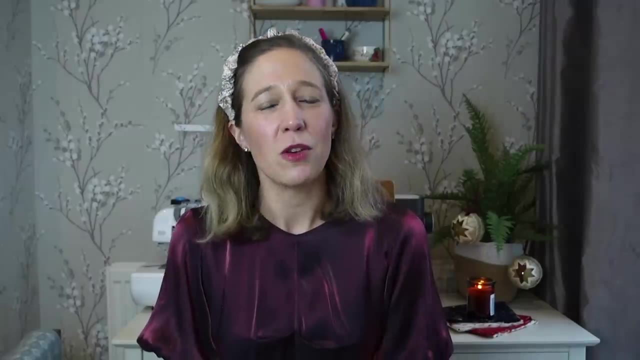 my children use these all the time. When we're sitting on the couch watching a movie, they are cuddling their hot water bottles. When they go to bed, they love to have their hot water bottle in there to keep them nice and toasty warm, Especially over the winter. right now, we're all trying to save. 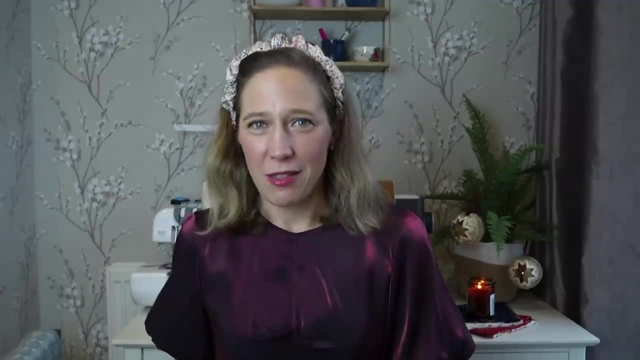 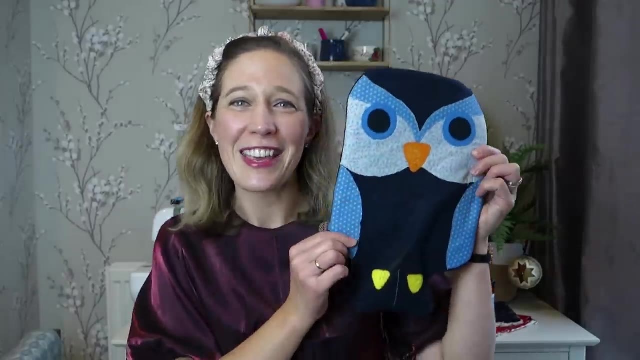 money. Hot water bottles are such a great thing to have, but they are so hot and I'm always worried about the burn risk. So what I did for my children was I made these hot water bottle covers, and these are from a pattern by Twig and Tail. Now there are lots of different animals. 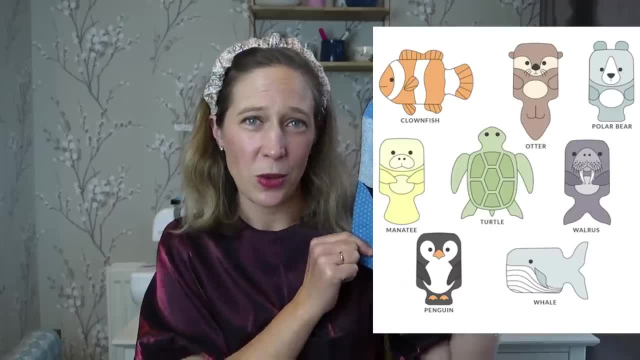 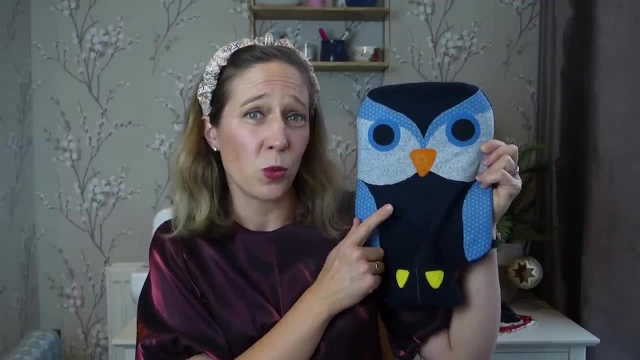 there are lots of different sea creatures and they are just so cute. So this is the one I made for my eldest son, and this is an owl made up of some scrap fabric I had from making his coat. So this is a boiled wool which really insulates and keeps the hot water bottle nice and warm. 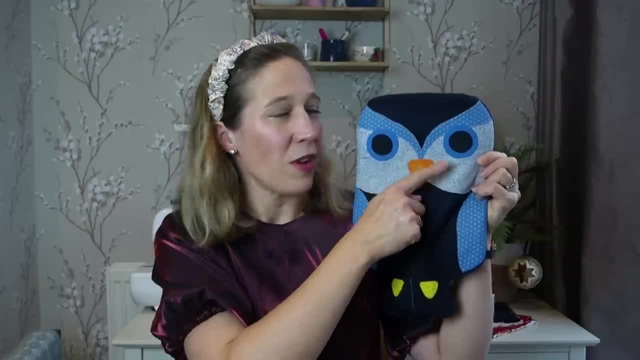 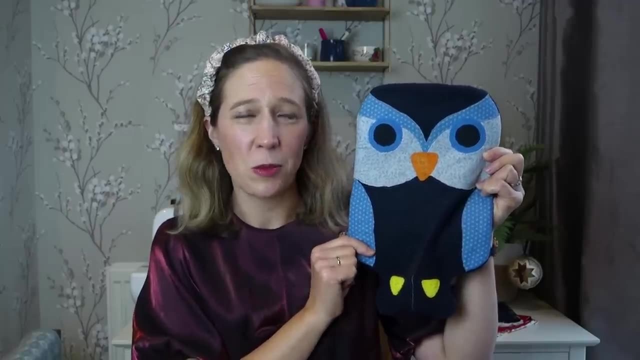 and keeps him from getting burnt. And then I had these fabrics just left over in my stash of fabrics and I used some bonda web and then I stitched them on, So it came together super quickly. and then at the back you've got a little opening so that you can easily fill the hot water. 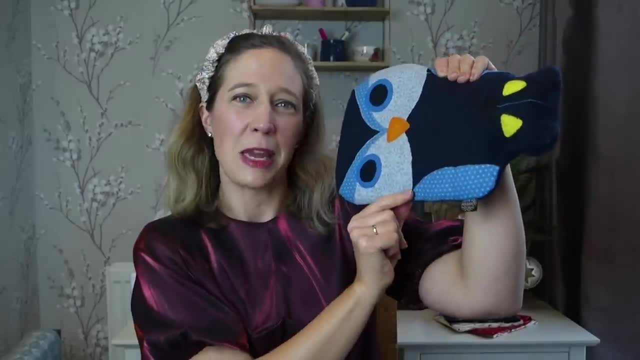 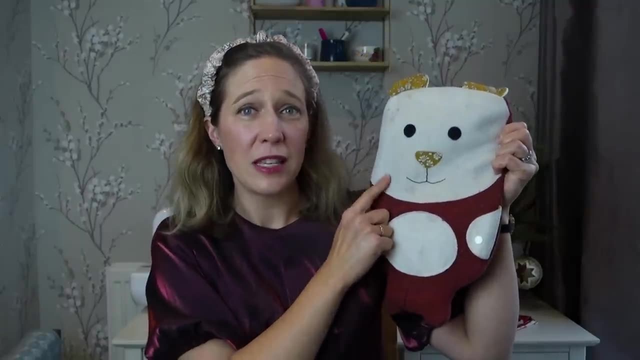 bottle and I added a little rosy cheeks label which says made by mummy. And for my second son I made a little bear, and this one again was made up from scrap fabrics. This was a fleece that I used to make a dressing gown for my children, and then a wool from a jumper that I had been. 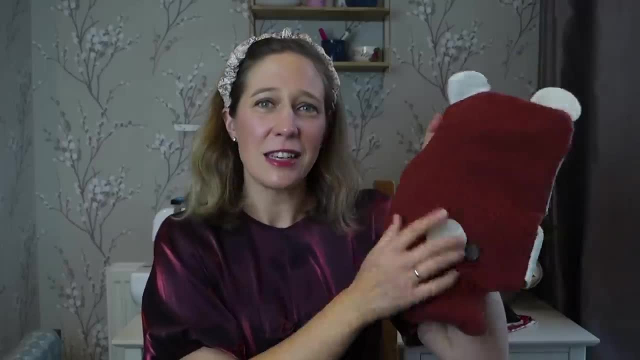 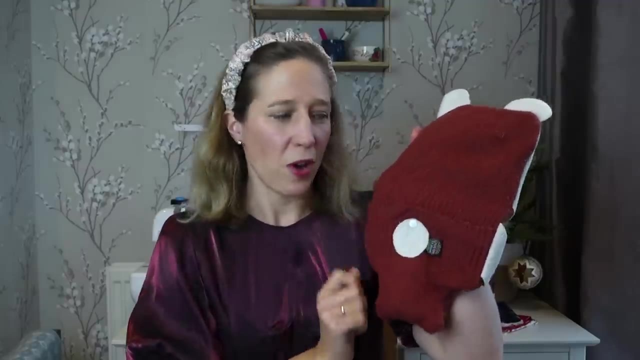 given by someone who was throwing it away. So I repurposed that and I used the edge of the jumper for the opening here of the hot water bottle to make sure that the hot water bottle was not that it didn't fray, I just used a popper to close them. so they open and close, really, really. 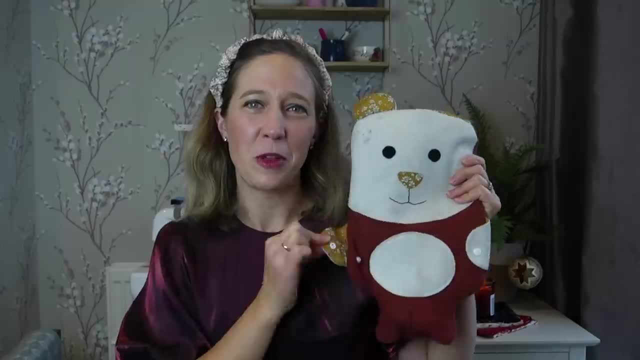 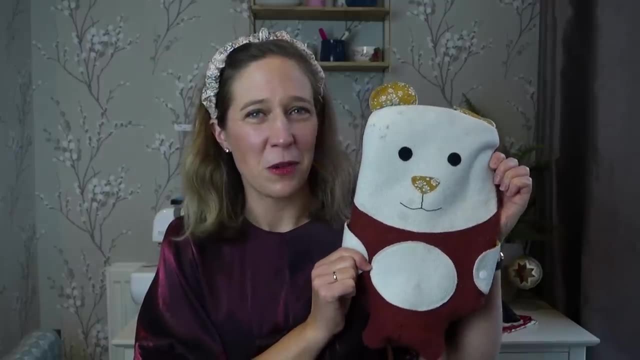 easily. And then this one is super cute because it has little poppers for the pores They can open and shut. so my son really enjoys playing with this hot water bottle cover, as well as obviously using it to keep himself warm. So this year I'm hoping to make one for my daughter, because she's just got to the 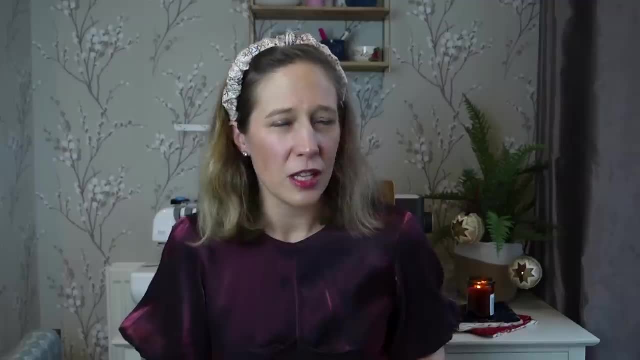 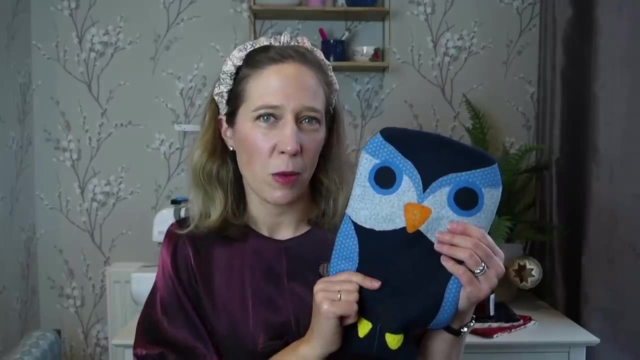 age where she's noticing that her brothers have hot water bottles and she does not. So, again, I made her a coat a few years ago in a similar boiled wool, but in a pinky colour. So I think I will use that for the base of her sweater. So I'm going to show you what I've made. So I'm going to 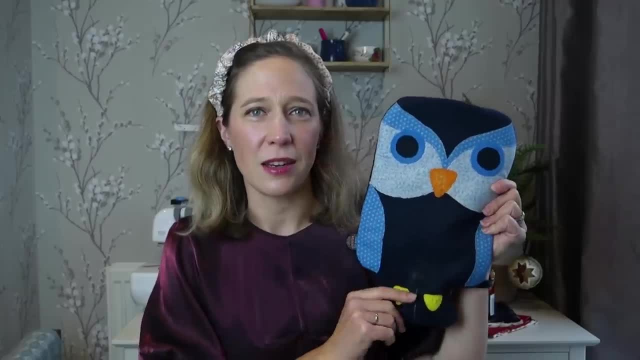 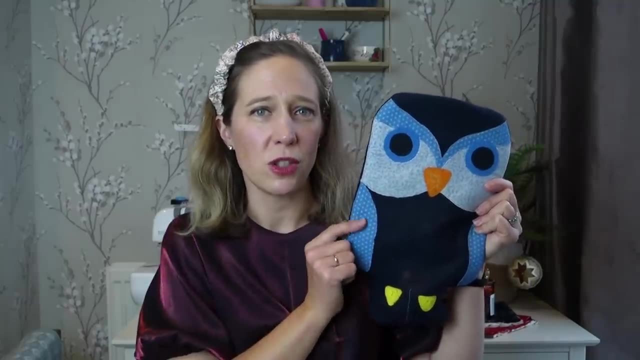 show you her hot water bottle, and I'll definitely be using this pattern again to make a cover. Twig and tail patterns are fantastic. The instructions are great. There's very clear photographs. If you've never done any sort of applique or patchwork before, you don't need to. 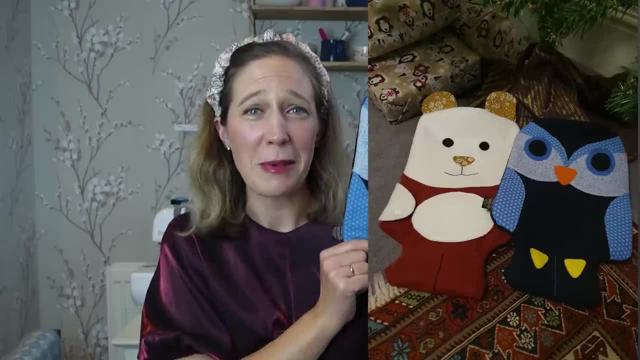 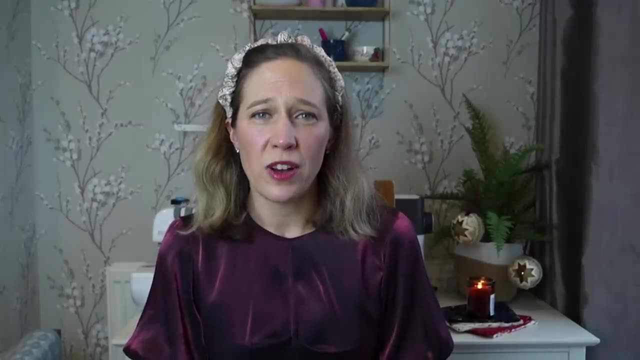 worry, It comes together beautifully, The instructions are fantastic and it just makes the cutest gift for children. The next idea I have is by one of my favourite children's pattern companies and that is Below the Corphi. Now, this is a New Zealand pattern company and Sophie has. 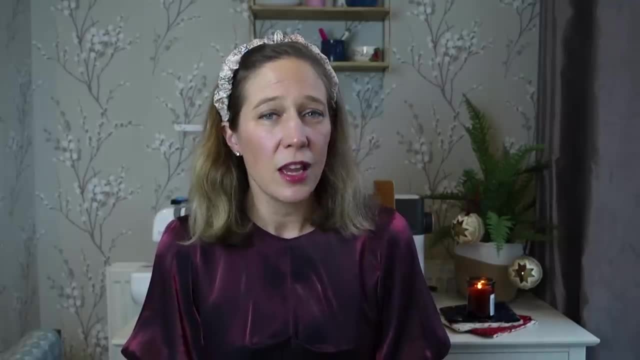 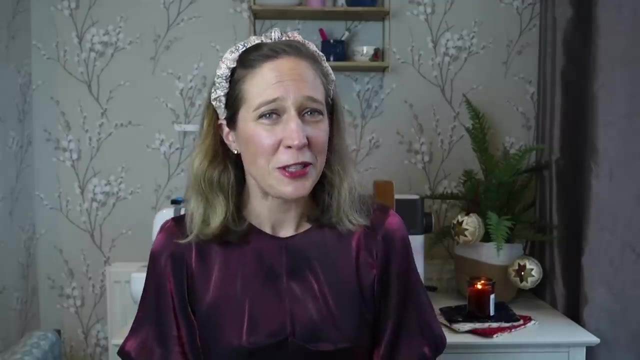 got some beautiful patterns for children, So I'm going to show you what I've made. So I'm going to show you the pattern over on her website. She also has some great gift ideas over on her website as well, So do go and check it out. She has a really cute animal purse that you can make for. 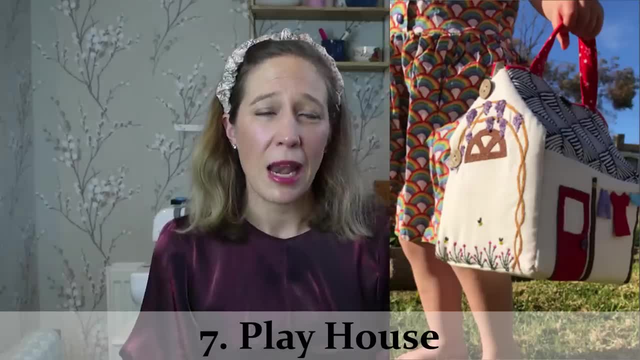 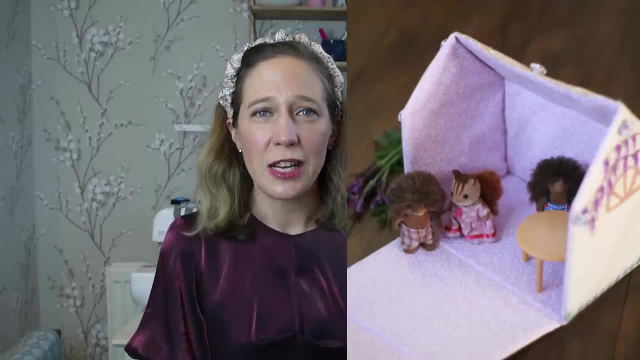 little girls in your life. But she also has this amazing playhouse, which is what I want to share today. Now, this playhouse, you can again make from scraps of fabric. You can decorate it however you want for really fantastic, open-ended play for your children. I think I saw some that had been. 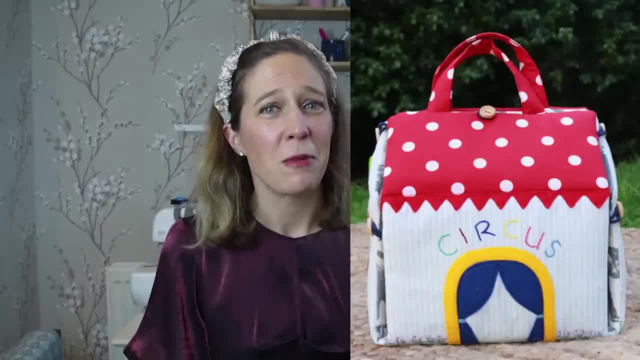 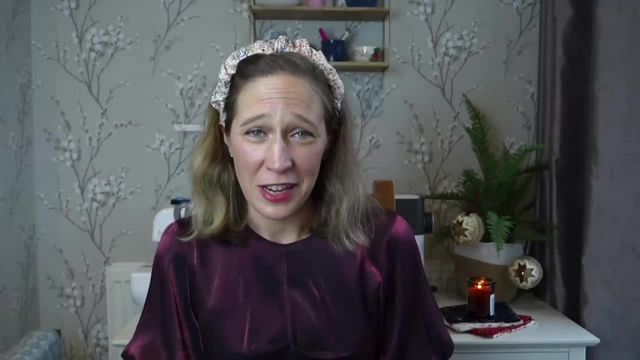 decorated as little houses, some as circuses, some as firehouses. You could really use it for boys or for girls and decorate it in any way that you like and use any fabric that you like. Now on the Below the Corphi website, when you buy the pattern, you can also buy the plastic inserts to use to. 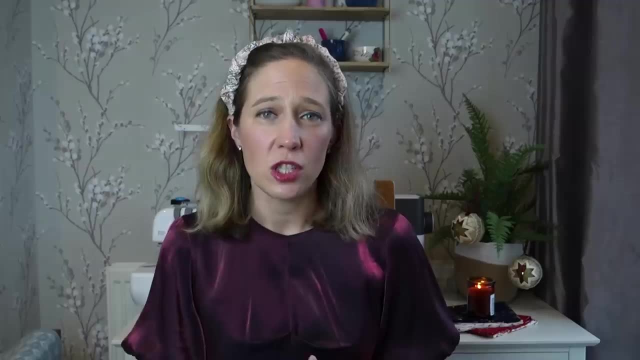 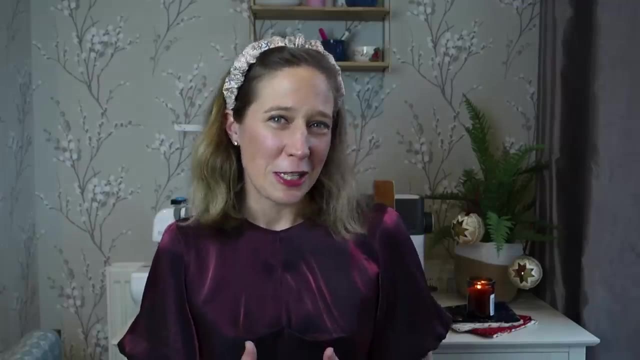 strengthen the walls of the house. But she also does have suggestions for what you can use and where you can get that. But I just think this would make such a great toy for children, especially when you live in London and there's not a great deal of room in our houses for gorgeous big dolls houses. 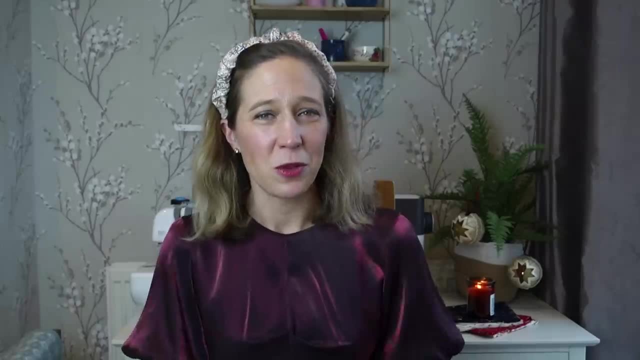 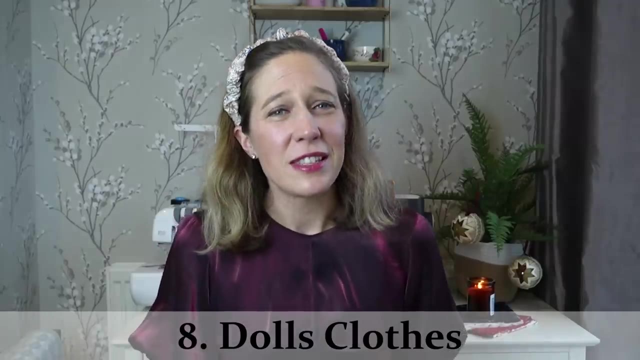 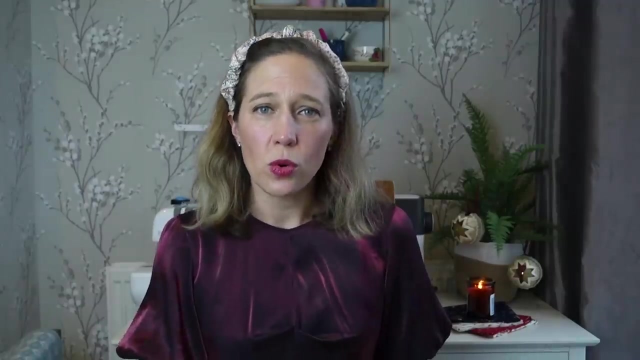 This would make such a cute little dolls house or a playhouse for children, and it's a great idea for a gift for fantastic open-ended play. Now my eighth idea is another one for children and this is some dolls clothes Now. I bought a pattern by Wild Marigold Patterns and it included all sorts of 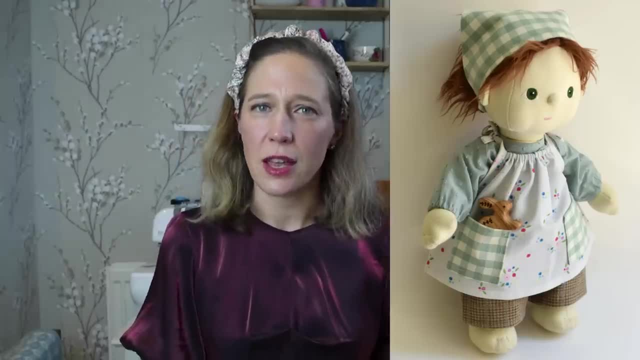 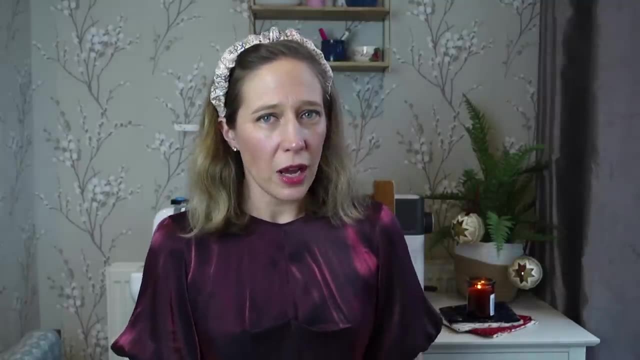 dolly clothes, from bonnets to dresses and trousers and shirts and nappies- All sorts of things that you can make for your dolls- and she has patterns for different sizes of dolls. So if you'd like to make some dolly clothes and you just want a pattern so that you can easily make something, 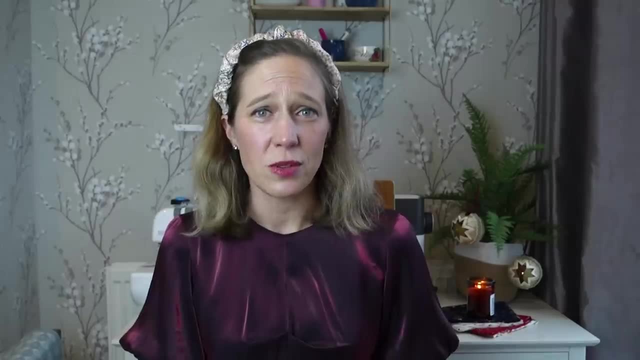 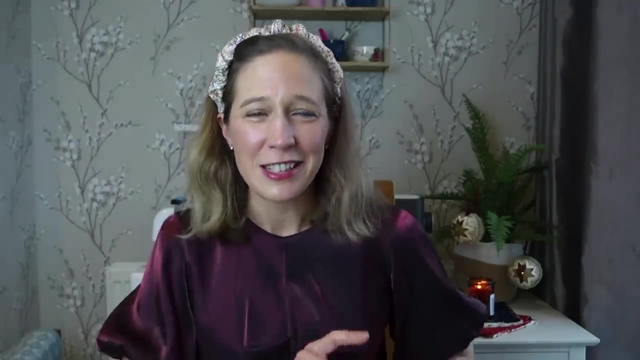 this is where to go. I have found the pattern really easy to use Again. it's great for scraps and it comes together beautifully. It's so easy. a child could do it and in fact, this is what my middle child, my five-year-old as he was then. 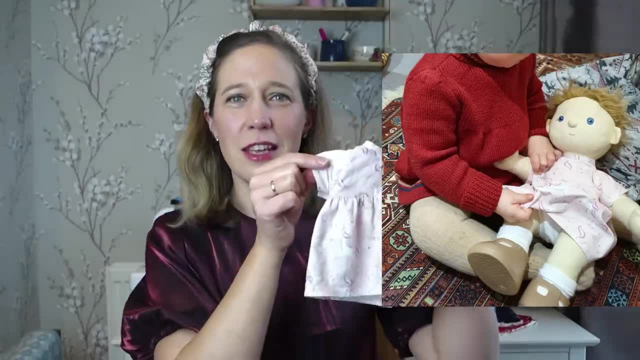 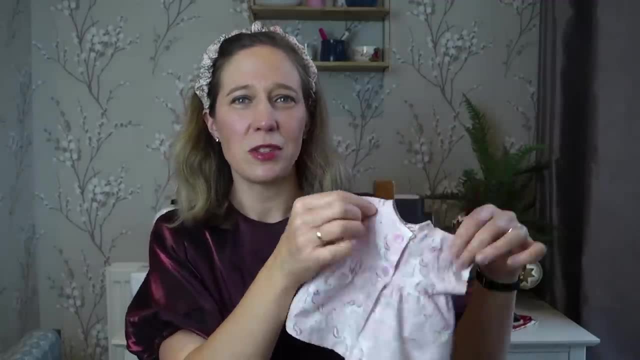 made for his sister for Christmas. And here's the little dress he made for her dolly. It was just made in some unicorn fabric that we had left over. Now I did help a bit with the sewing, but he did some of the cutting out. He pushed the foot pedal on the machine, so he felt quite accomplished. 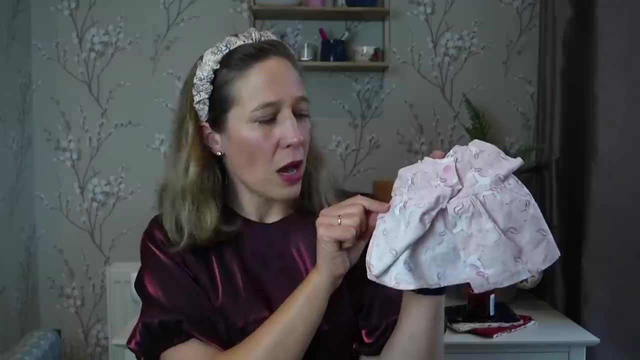 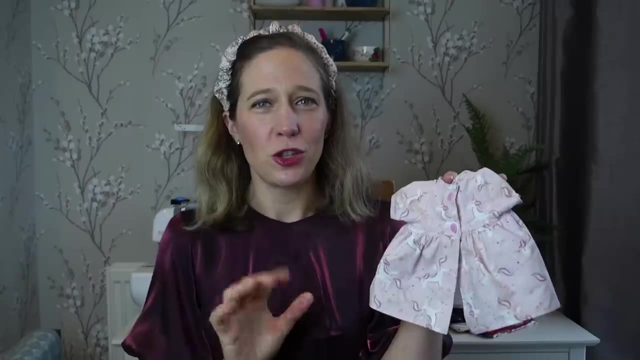 at the end, and he helped to squeeze these poppers on as well, which he loved. So a really lovely design. It's finished really beautifully because obviously children are taking these on and off their dollies all the time, So you do want it to be nicely finished so that it lasts for a long time. 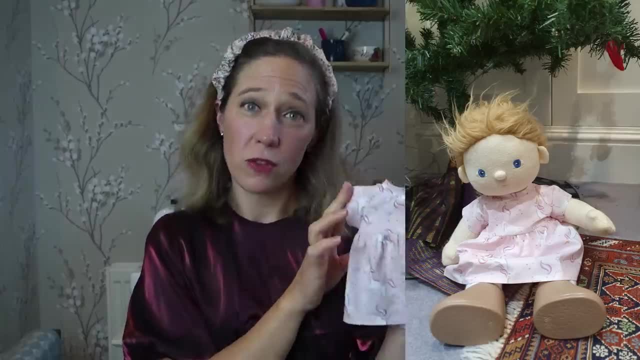 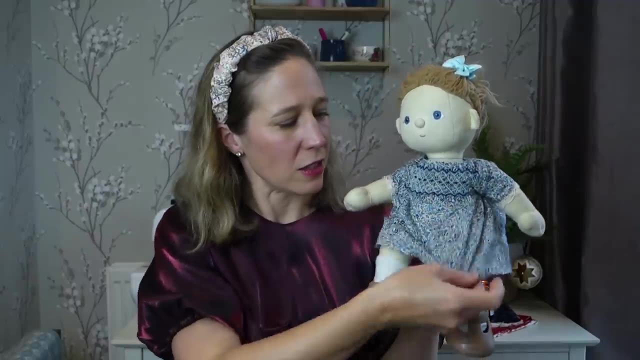 and this has been well used and played with lots. It's off the dolly at the moment, as you see, but on dolly is another one that I made, and I made this for her birthday present. actually, This little dress from a scrap of the liberty I had left over from making her birthday dress And 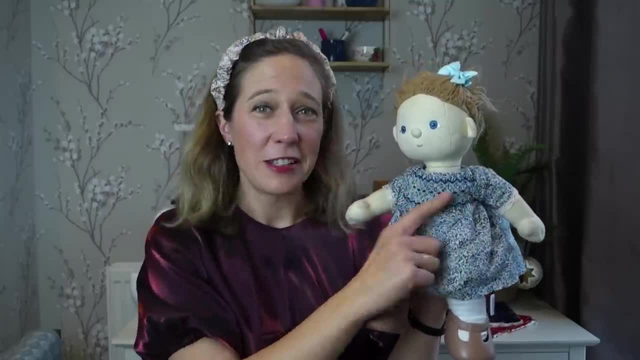 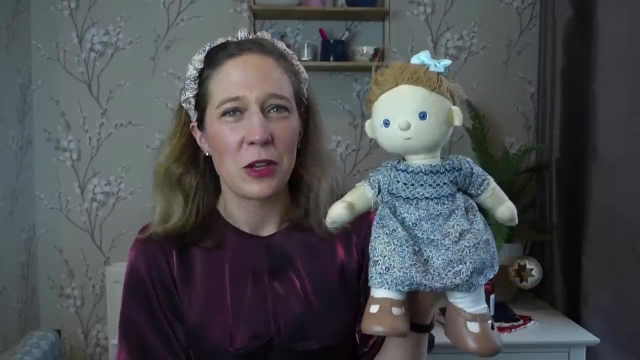 again. it just came together so easily and you can personalise them as well. I decided to smock this because I did, and I also put lace on the sleeves just for fun, and she loves this one as well. She puts on dolly a lot, so that's my other idea for sewing for children, So the pattern is great. 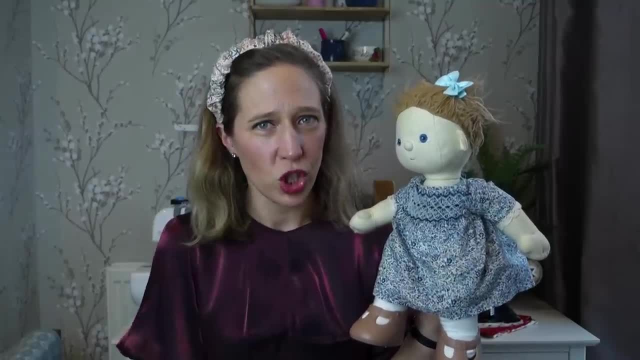 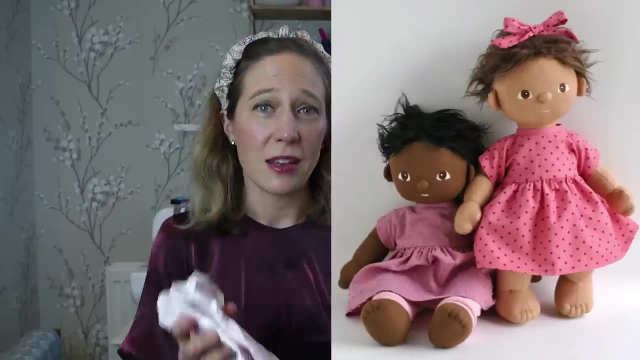 because it does have this dress, but it does also have trousers, shirts, jumpers- I think there's, like I said, bonnets and hats, all sorts of different items of clothing. I just happened to have made the dress and my son made the dress, because it was a pretty easy, straightforward sew. My ninth idea that I've seen on Pinterest and I just think looks so much fun for children is fabric car play mat- Again, a great stash buster. Use all sorts of different kinds of fabrics to piece this one together and you'll end up with such a great toy- Now the one that I've linked. 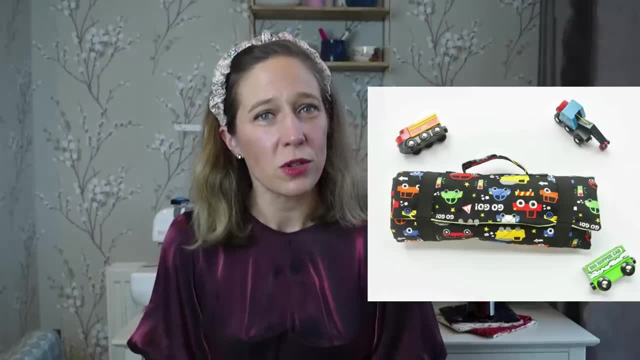 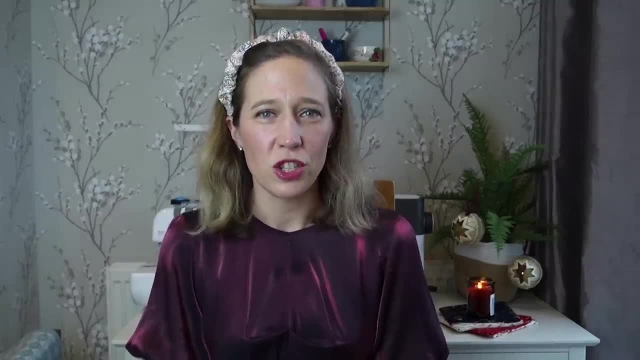 below is one that you can roll up and take with you wherever you go to restaurants or if you're travelling on a train or a plane. over Christmas, This would be a fantastic one to take with you, and then you can just unroll it and the children can have, hopefully, some lovely open-ended play. 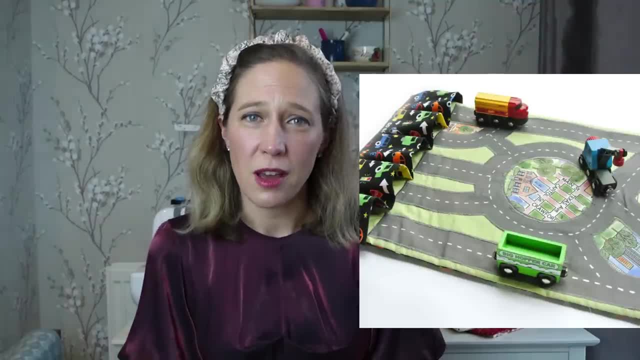 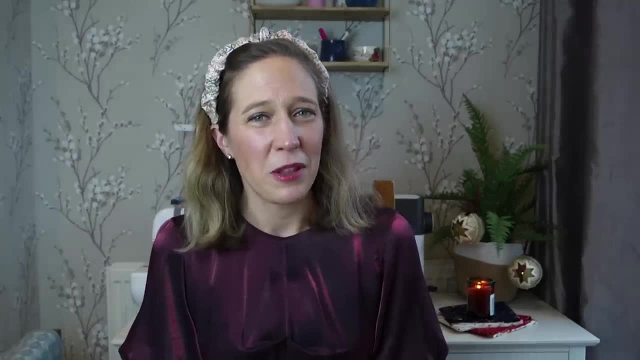 with this toy Now, the one I've linked below has slots where you can put the cars in to store them, and great for travel, and I just think this would make such a fun gift for children to play with over Christmas. The last gift I'm going to share with you today- gift number 10, is Christmas. 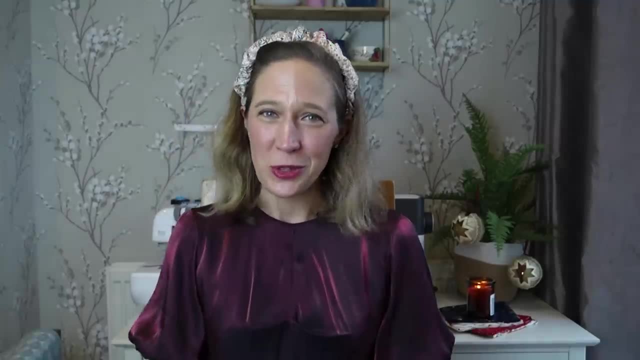 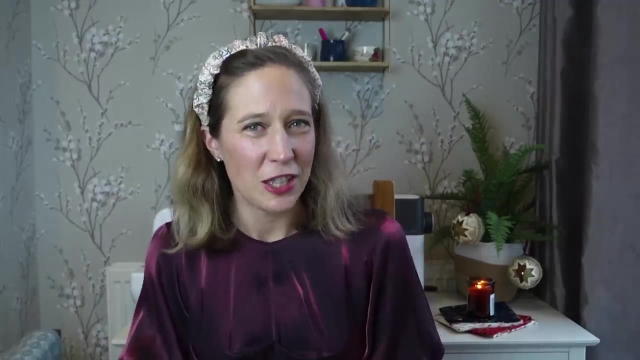 pyjamas. I had to include it, didn't I? I mean, we all sew these for our children. We have a tradition in our house where, on Saint Nicholas Day, they wake up, they find coins in their shoes, they find a fresh set of Christmas pyjamas to wear and they love it. We like to give it to them early on. 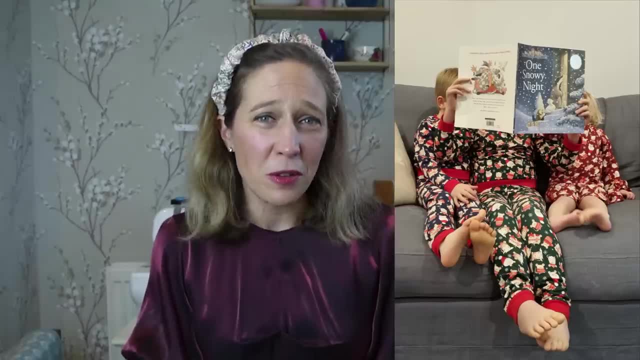 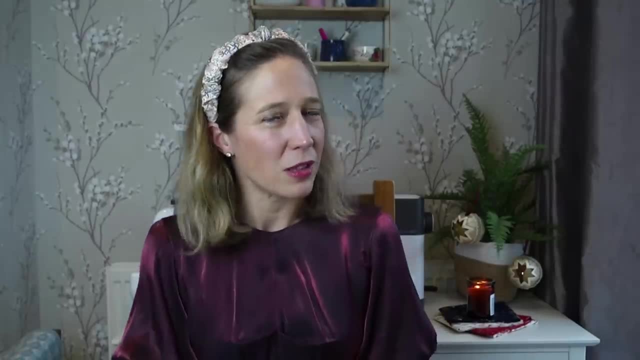 in December, on Saint Nicholas Day, because then they get to wear them for the whole of the festive season and they just adore wearing their Christmas pyjamas. Often they get changed to them the minute they get home from school, and with the weather as frightful as it is at the moment, who can blame? 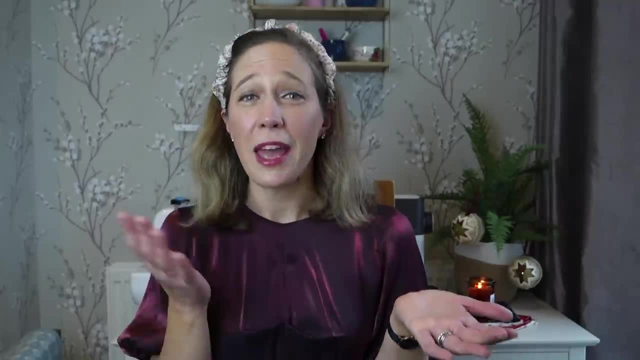 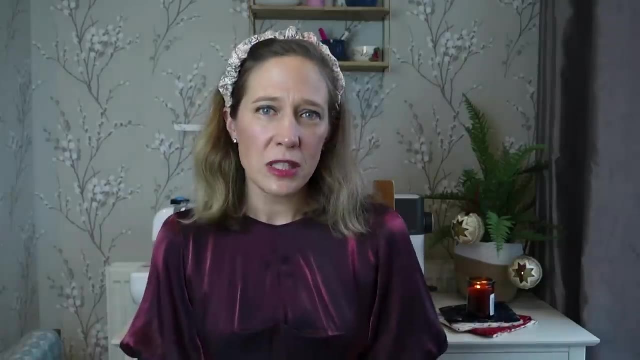 them. So I've got some pyjamas for Northern Hemisphere people and for Southern Hemisphere people. There's who doesn't want Christmas pyjamas wherever we are in the world, And these patterns are all free. The first ones I'm going to share with you are from a website called Sew Simple Home. 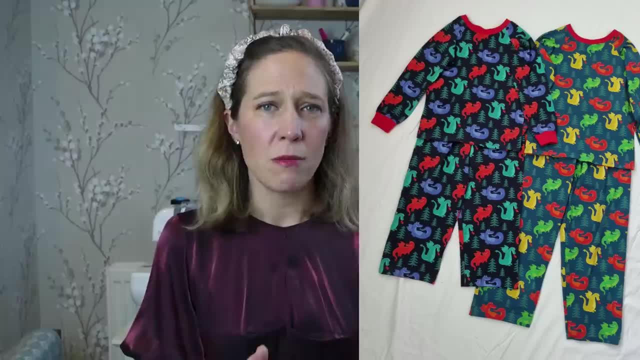 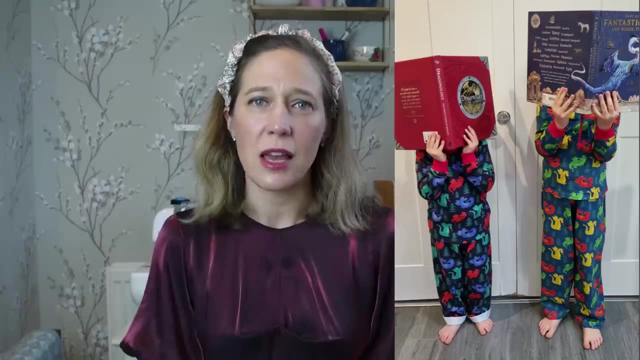 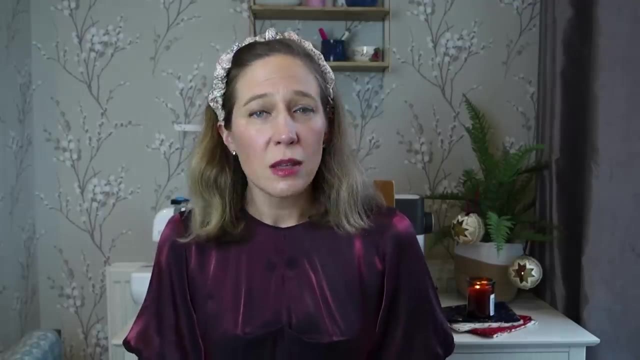 There's a short sleeve or a long sleeve raglan t-shirt and some long trousers. Now, my children don't have a cuff and that don't come in at the ankle. They like them to be loose. and these are perfect And they were such a quick and easy sew and they are free. So that's the pattern that I'm. 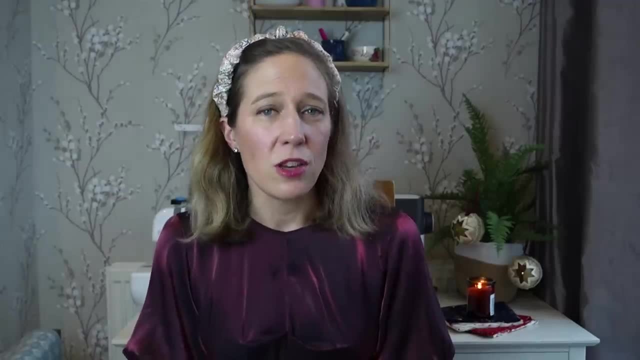 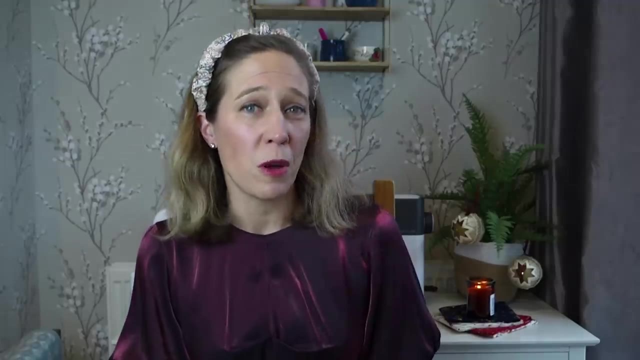 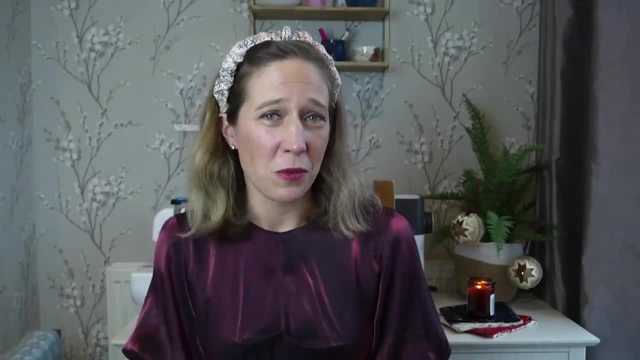 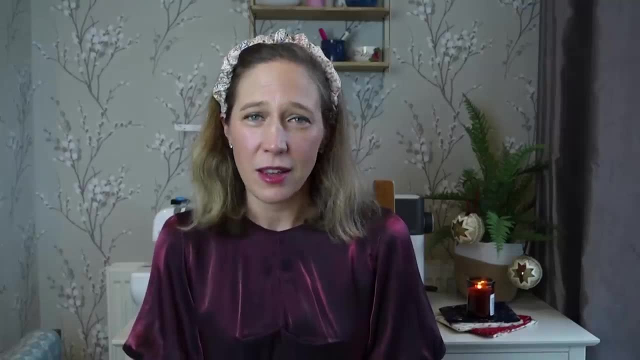 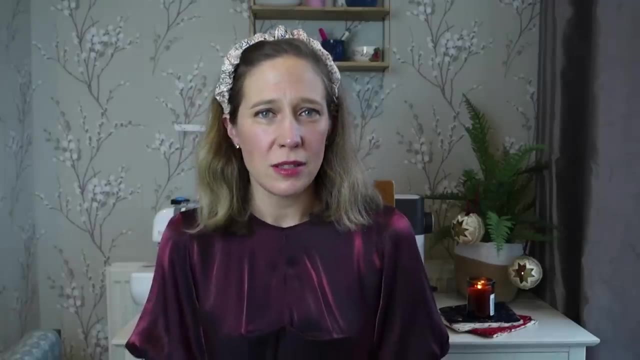 Yourself D-I-B-Y Patterns and it's the Anything But Basic A-B-B t-shirt. Now this again comes as a short sleeve or a long sleeve t-shirt, and the best bit about this pattern is it comes in a slim fit or in a regular fit, so it really will fit any children, which is great, And again, it's a free. 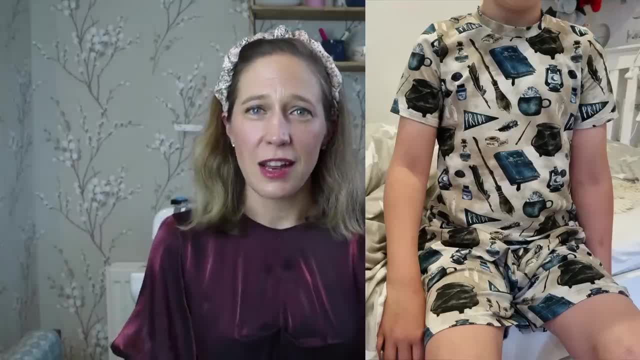 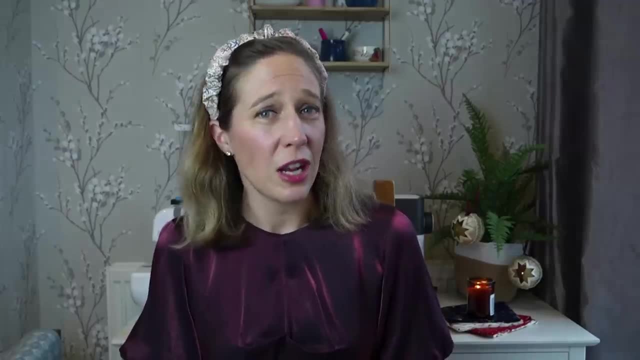 pattern. So this is what I use when I make them summer pyjamas, and it's a really good pattern. It's such a lovely little set. My boys wore their summer pyjamas all the way through the summer in this lovely cotton jersey that I bought from Jelly Fabrics. But this year I'm so excited about 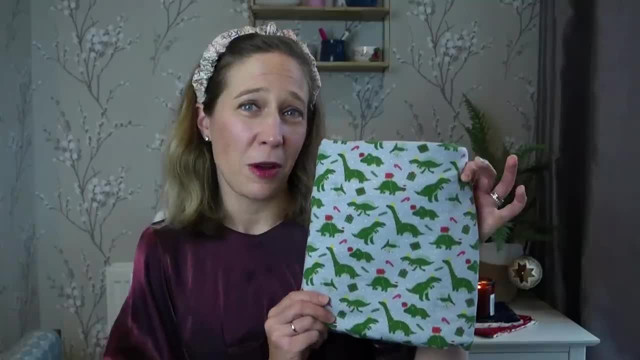 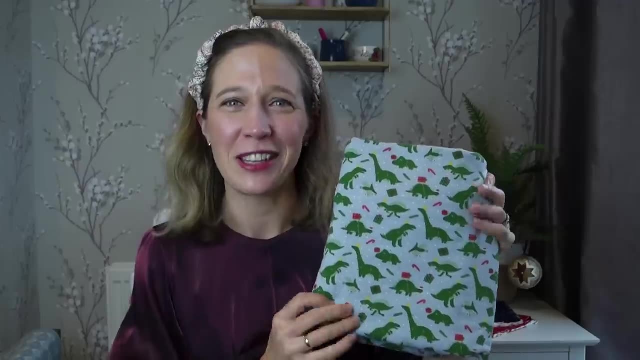 their Christmas pyjamas. I have bought this fabric from Empress Mills and it's Christmas dinosaurs. because dinosaurs and Christmas, I just think that's perfect. So this fabric will be for one of my boys. and then I've got a green fabric, but you can't see the dinosaurs quite as clearly. 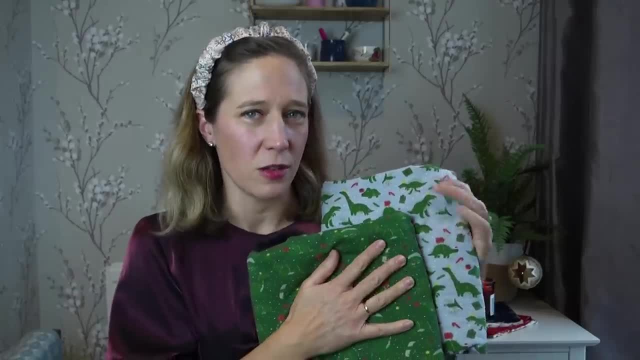 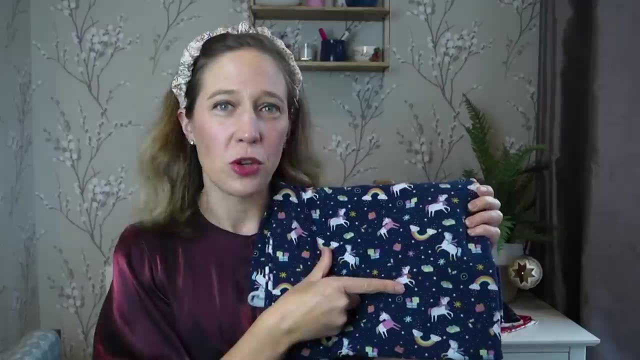 on this one. But I've got a green fabric which also has a green fabric on it. So I've got a green fabric which has the Christmas dinosaurs on. So these will be for my boys And then for my little girl. I have got this unicorn Christmas fabric. It's got unicorns, it's got little gifts, So not 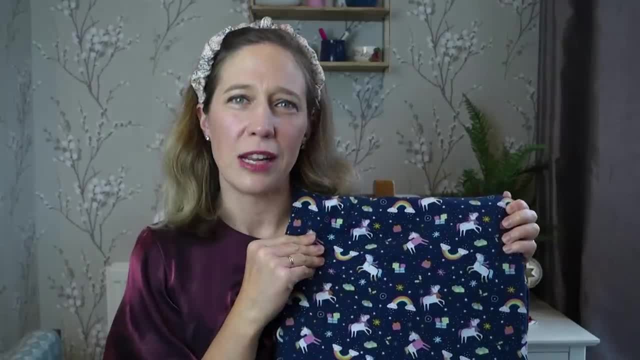 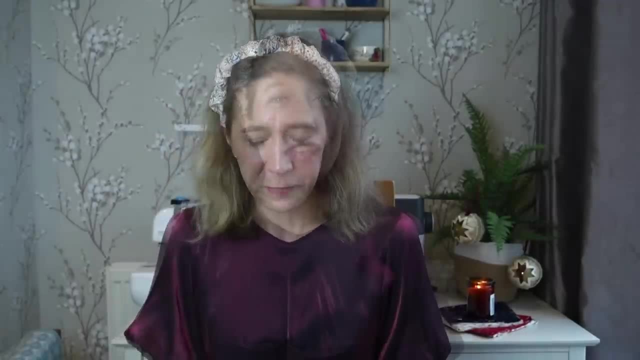 overly Christmassy, but just Christmassy enough that I think she'll really love that. I mean, who wouldn't love unicorn pyjamas? I'd love unicorn pyjamas, But I don't think there's enough fabric for me as well as for her. So, to finish off, I thought I would just quickly share what I'm. 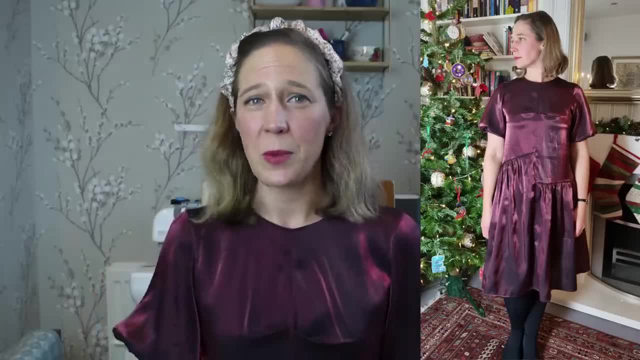 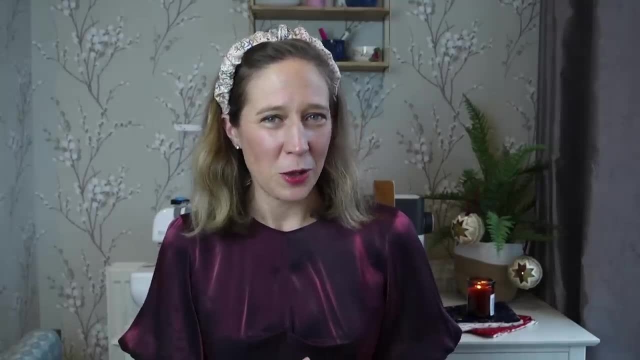 wearing today. This is a dress that I made last year for Christmas, but I will definitely be wearing it again. I do lots of singing and playing at carols and I'm going to be wearing this during the Christmas season, So this one will get lots of wear during the festive season, not just.